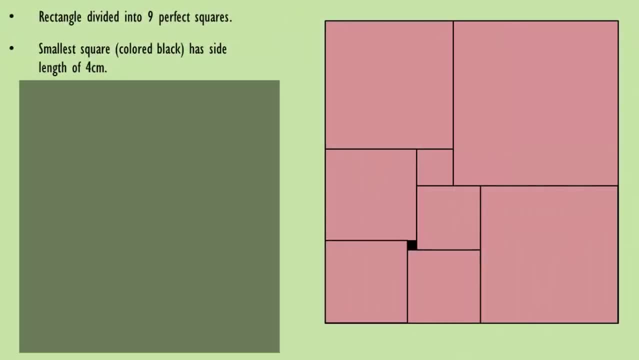 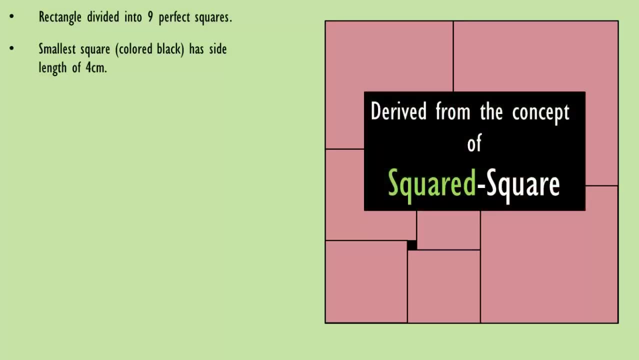 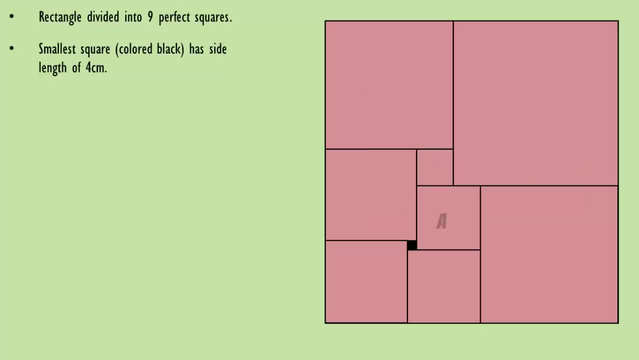 I'd like to thank Krishna for sharing this very unique math puzzle. It's derived from the concept of squared square, on which I'll post a detailed video in near future. Let's see how to solve this problem. Let's name the remaining 8 squares from A to H. 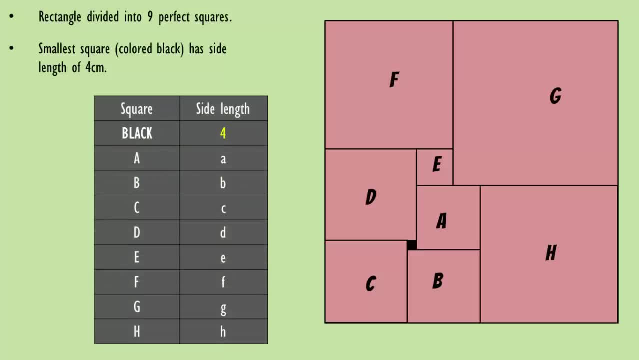 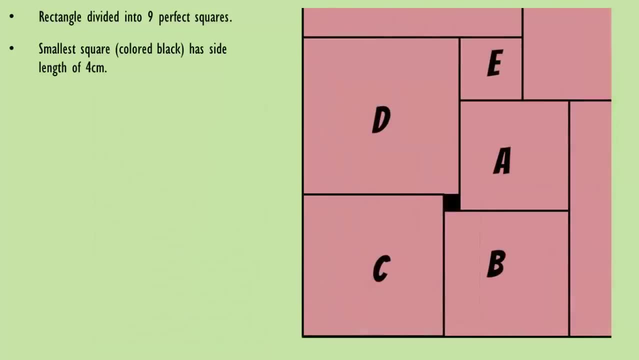 You can name them in any order, And let's denote their respective side lengths in the lower case. Now, the only possible square to start the calculation with is the black colored square. Side length of square B should be equal to the side length of square A. 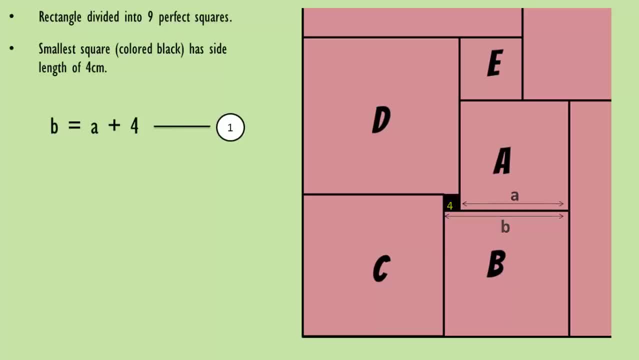 plus 4.. And this is our equation 1.. The same way we can get the equation C equals B plus 4.. And if we substitute the value of B from equation 1, we get the equation C equals A plus 8.. 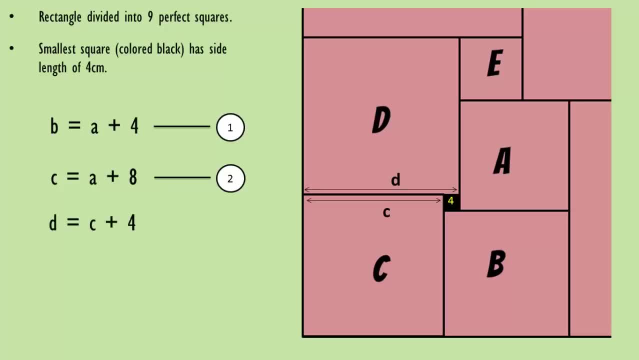 Now D equals C plus 4.. Substitute the value of C. We get D equals A plus 12.. After 3 equations we have managed to indirectly compare side length D with side length A. But we can also directly compare D with A, as shown. 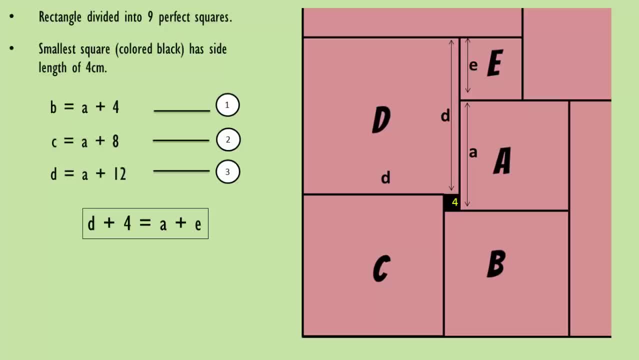 So D plus 4 is equal to A plus E. From equation 3, we have: D equals A plus 12.. So we get the value of E And that's 16 centimeters. Now let's make some more equations. F is equal to: 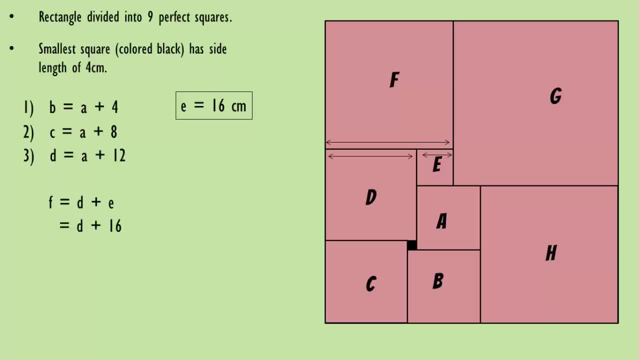 D plus E. Substituting the values gives us the equation F equals A plus 28.. G is equal to F plus E, So we get G equals A plus 44.. H is equal to A plus B, And that's equal to 2A plus 4.. 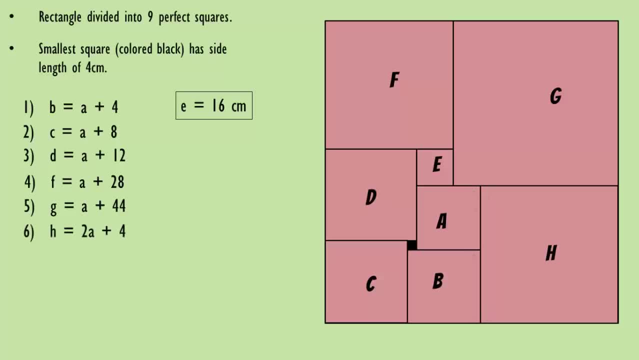 Now, as we have covered all the individual squares, it's time to make one or more equations using the side lengths of money, For example, we can use the formula for the value of D to solve for the unknown variables. Based on the equations you make, it may take several attempts to find the value of a variable.